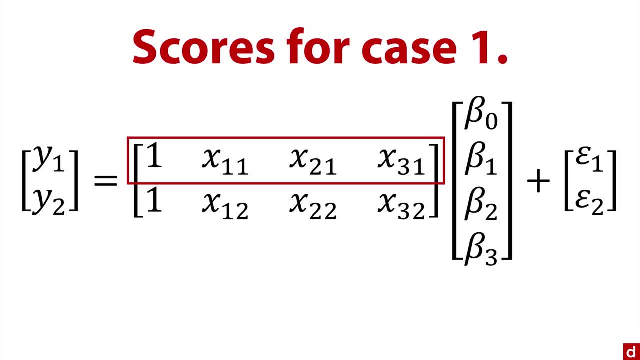 is to indicate that it's for person one. Below that are the scores for case two, the second person, And then over here in another vertical column are the regression coefficients. That's a beta there that we're using, And then finally we've got a tiny little vector here at the end. 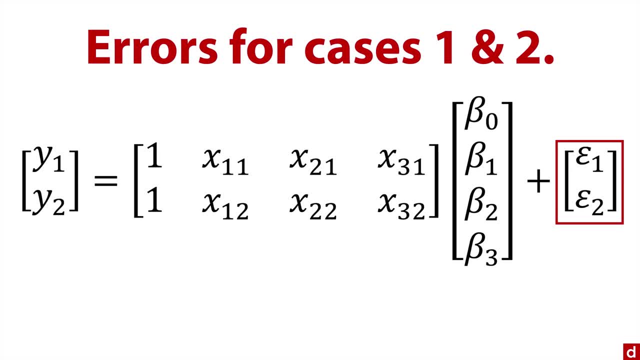 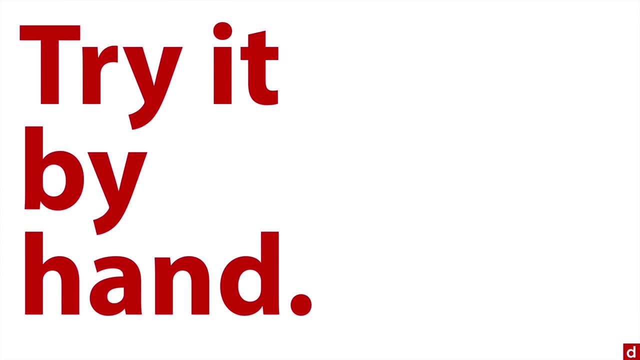 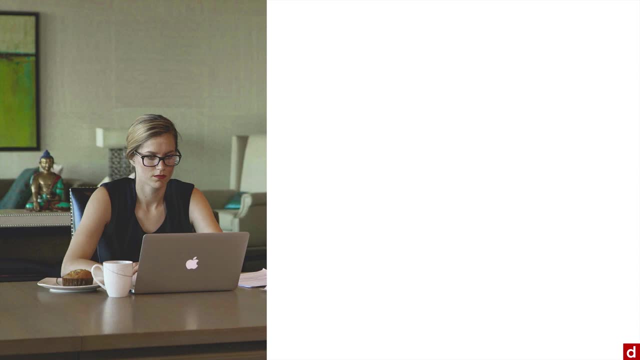 two fictional people. This will be fictional person number one. we'll call her Sophie, we'll say that she's 28 years old and we'll say that she has good bargaining skills of four on a scale of five and that she works 50 hours a week and that her salary is 118,000.. Our second: 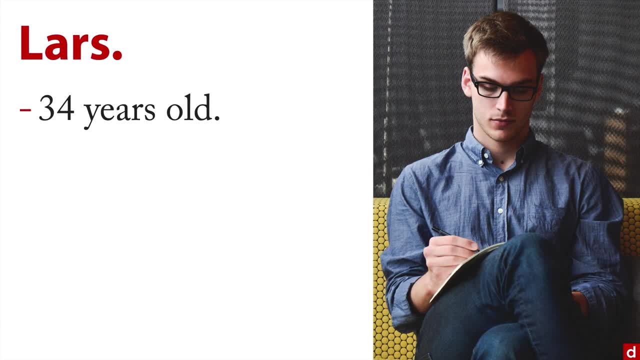 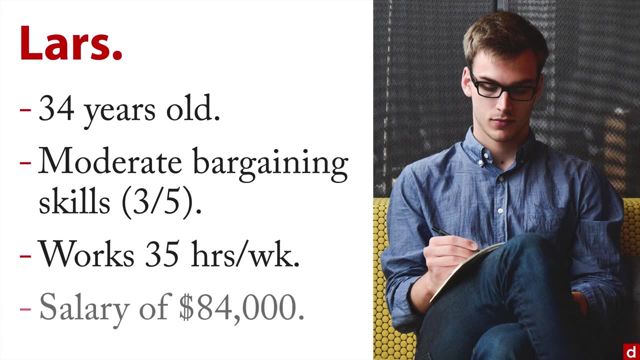 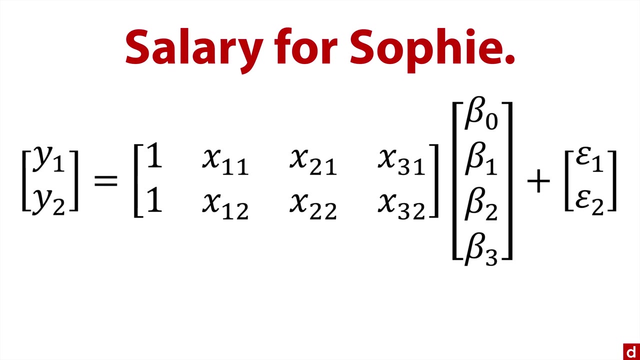 fictional person. we'll call him Lars and we'll say that he's 34 years old and he has moderate bargaining skills. three out of five works 35 hours per week and has a salary of $84,000.. And so if we're trying to look at salaries, we can go back to our matrix representation that we had. 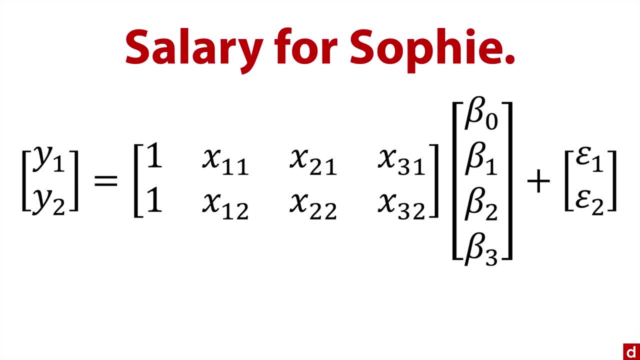 here with our variables indicated with their Latin and sometimes Greek symbols, And we're going to replace those variables with actual numbers So we can get the salary for Sophie, our first person. So let me plug in the numbers here And let's start with the result here. 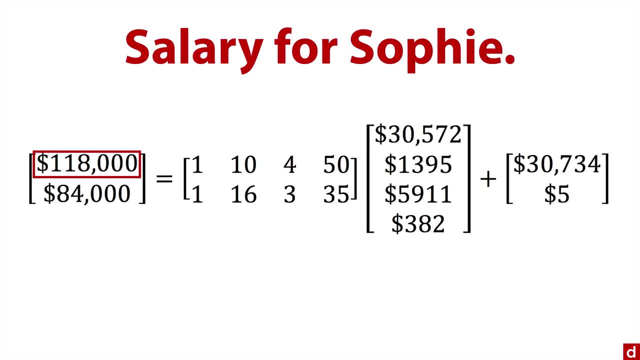 Sophie salaries: 118,000.. And here's how these numbers all add up to get that. And the first thing here is the intercept, And we just multiply that times one. So that's sort of the starting point. And then we get this number 10, which actually has to do with years over 18.. 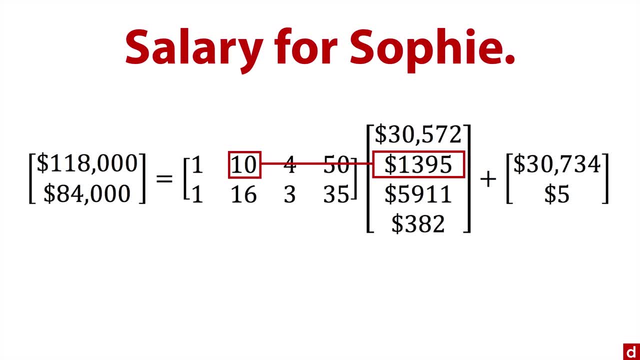 She's 28.. So that's 10 years over 18, we multiply each year by 1395.. Next is bargaining skills. she's got a four out of five And for each step up you get $5,900.. By the way, these are real. 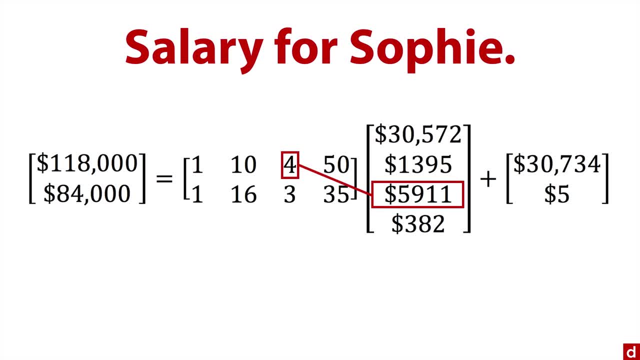 coefficients from study of survey of salary of data scientists, And then finally, hours per week. for each hour you get $382.. Now we can add those up and we can get a predicted value for her, But it's a little low. it's 30,000 low, which you may say well, that's really messed up Well.